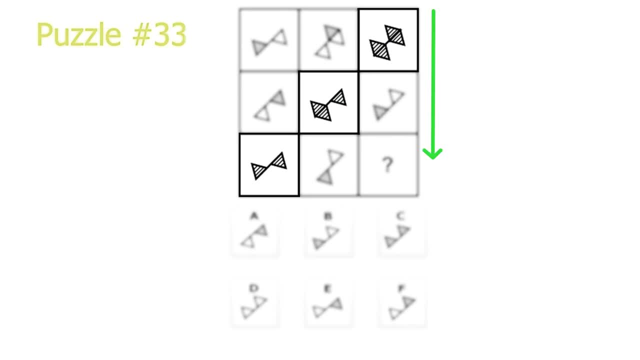 what changes when you move down on this diagonal. The second picture in the diagonal is just the first picture with the top right triangle gone, and the third picture in the diagonal is just the second picture with the bottom left triangle gone. So when looking only at this diagonal, you might think that the 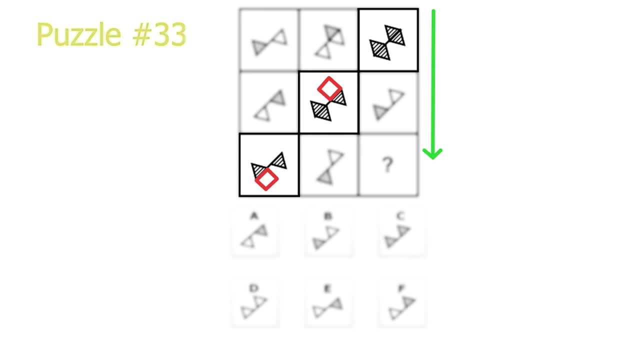 top right triangle disappears, and then the bottom left triangle disappears as we move downwards. Let's take a look at a new diagonal and see if it follows a similar pattern. I'll pick the red diagonal, since it has three pictures to base ourself on. Here we have a constant amount of triangles, so removing 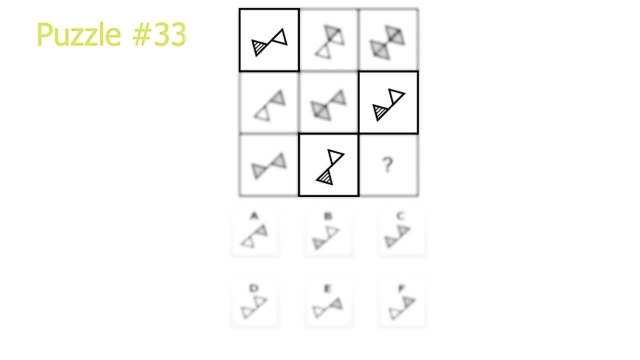 triangles, like in the first diagonal, won't work for this diagonal. For a new transition model, we can base ourself on this diagonal and describe a flipping effect To produce the picture in the second row using the picture in the first row. we just flip the bottom right triangle to the top right and to produce 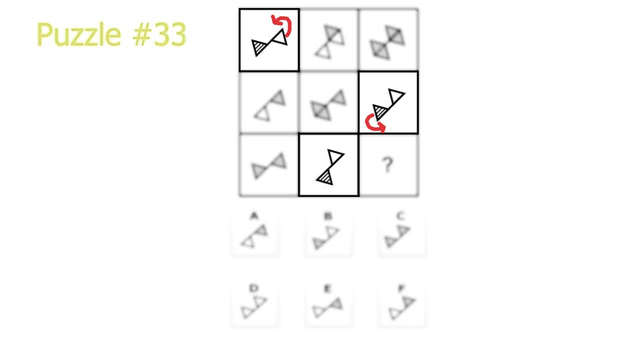 the picture in the third row. using the picture in the second row, we just flip the top left triangle to the bottom left. Let's take a look at the final green diagonal. We notice that the flipping of the triangles can also describe this diagonal. but here we have a new rule. If 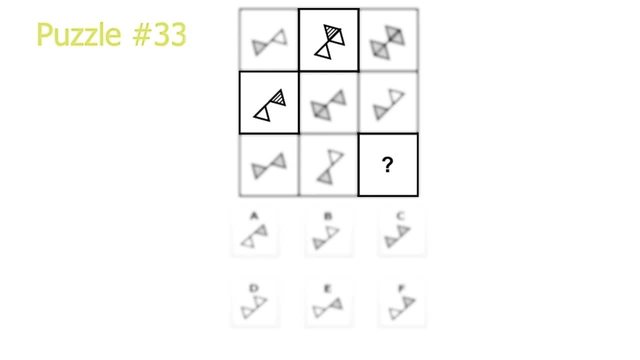 we flip a triangle on top of another triangle, then the triangle that gets flipped over shows instead of the original triangle. So to get the picture in the second row, using the picture in the first row, we just flip the top right triangle over to the bottom right and see that the striped triangle sits on top. 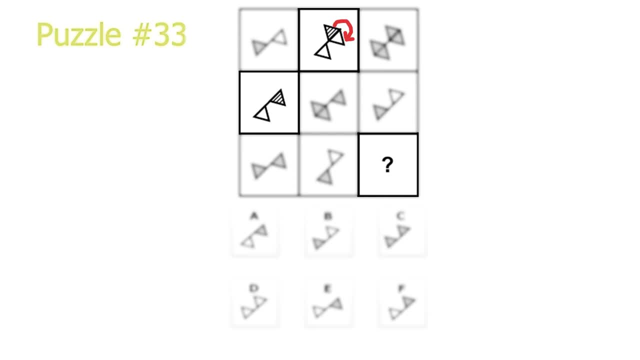 of the white triangle. therefore the striped triangle only shows. Let's go back to the first blue diagonal and try to use this flip transition. So picture 2 is just picture 1, with the top right triangle flipped over to the bottom right, and picture 3 is just picture 2, with the bottom left triangle being 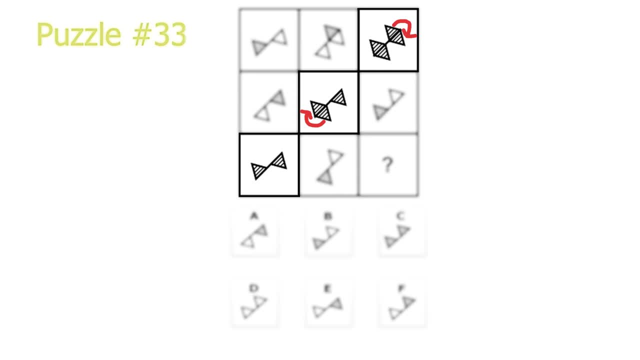 flipped over to the top left. This flip transition can describe every transition in this puzzle, from the top right to the bottom left- diagonals. But there is one problem: How do we decide which triangle gets flipped over First? let's take a look at the first row in order to see how we go from row one to row two. We